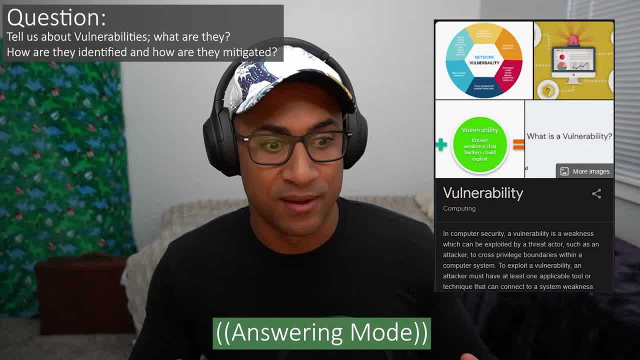 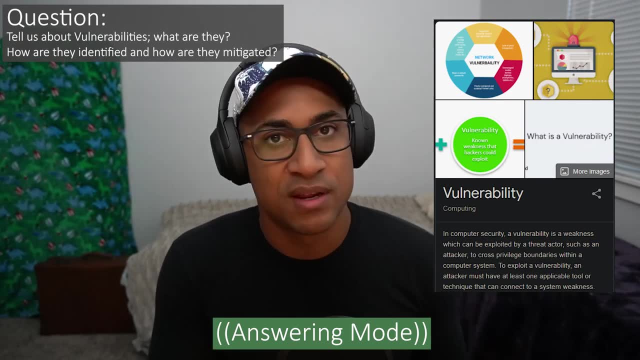 is just some kind of weakness in some system, whether it's like a physical, like location, can have vulnerabilities, or like a software can have vulnerabilities, or like a computer system itself can have vulnerabilities. it's just a weakness, um, in any kind of given entity, i guess. if you 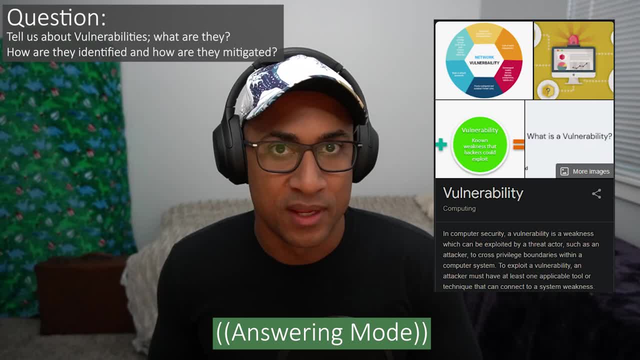 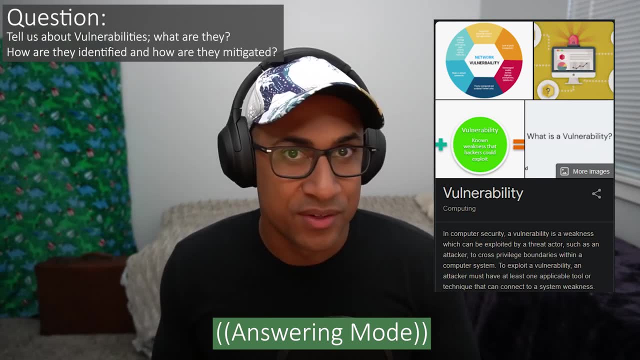 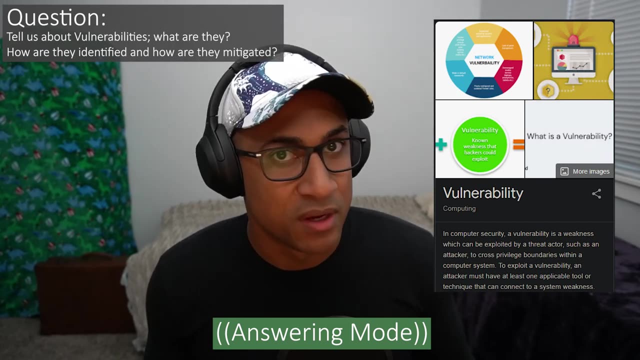 want to be really general about it. so an example of a vulnerability for a facility might be being built on a fault line where those earthquakes are being built above ground in a tornado zone, like something like this. or it could even be like the facility has like locks that were recalled by the manufacturer because like they don't work very well, or 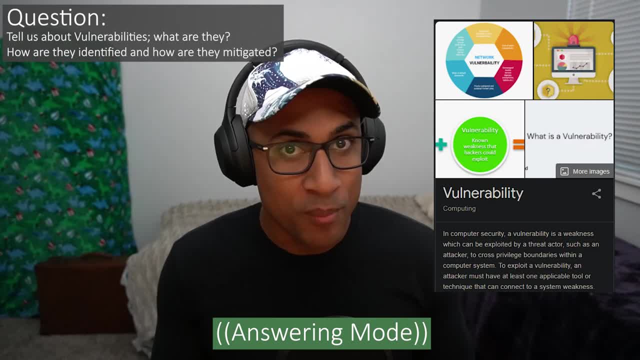 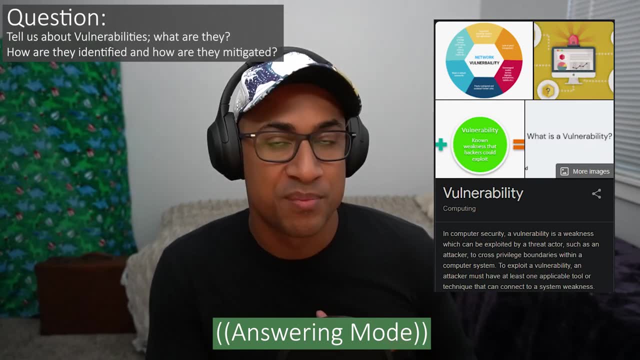 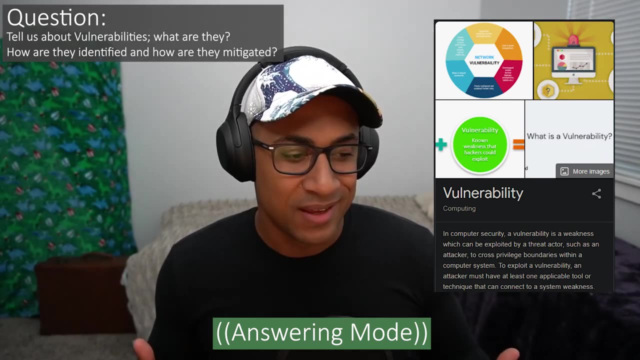 something like this, an example of a vulnerability on your home, like windows pc, for example, might be out of date software that's, you know, susceptible to buffer overflows or something like this. or you might be running insecure protocols like smbv1, um, or it could be could be like a misconfiguration. 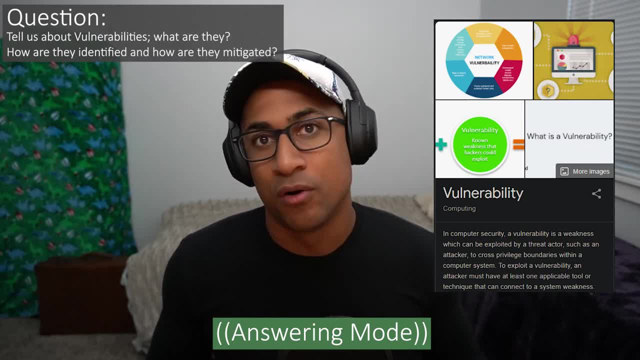 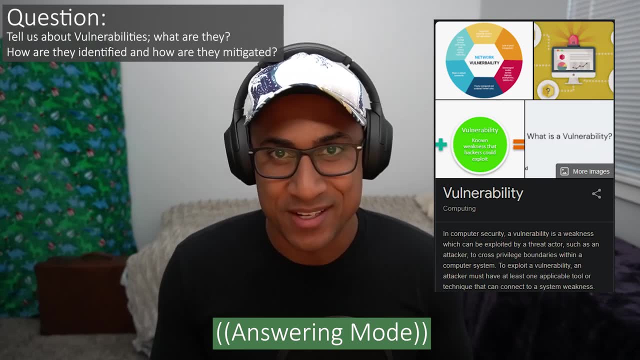 on your operating system or something like that. so it could be like a vulnerability on your operating system, like you have no password, for example, or there's no lockout policy so people can like easily brute force it. so to get the idea it's just like a general weakness in any kind of system or thing. 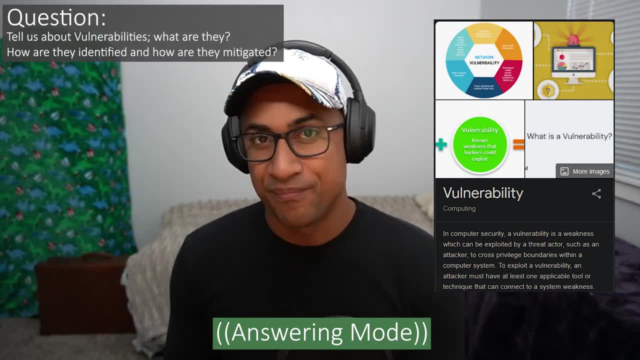 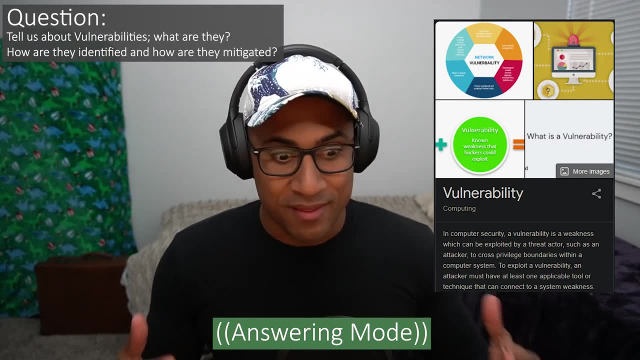 and vulnerabilities can be identified in like a lot of different ways. um, you can do some kind of manual inspection of the thing, whether it's like a building or computer system, like you can look at it and think about it and and find vulnerabilities that way. or you can use some kind of automated scanning software like nessus or 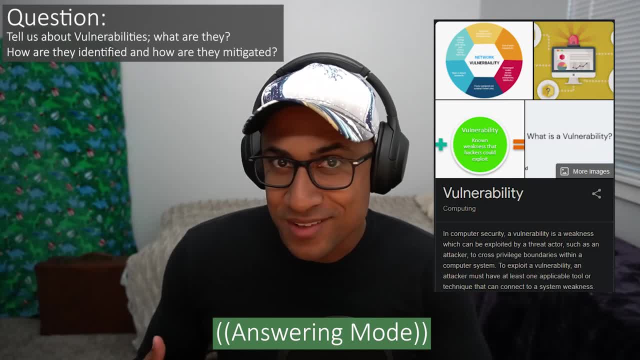 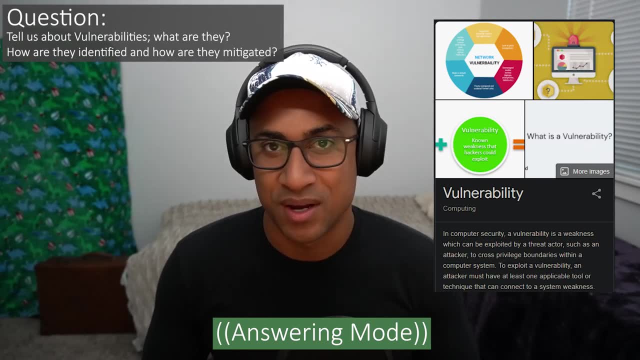 rapid 7, insight, vm or qualis, something like this. there's a lot of different ways to identify it, like manual or or automatic. you can use scanners, a lot of different software to to identify, and then vulnerabilities are mitigated in like many different ways, like, depending on you know if it's. 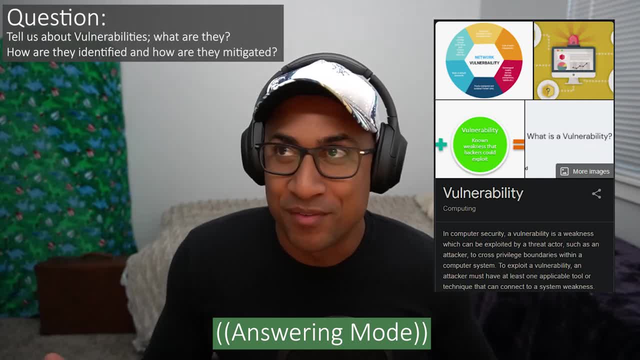 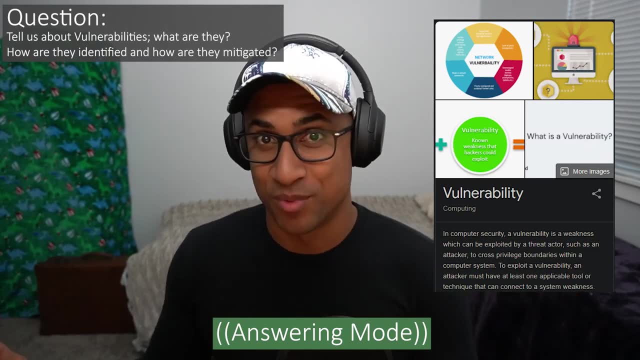 going back to the data center, right, if the data center is like built above ground in a tornado zone, like the only way to like really mitigate that is like maybe build it underground or like move it right to somewhere else or replace the locks on it and like for your 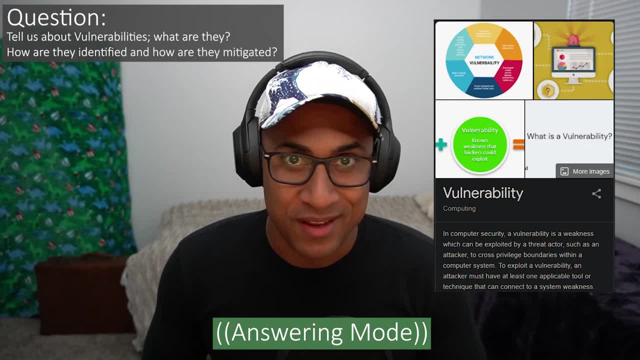 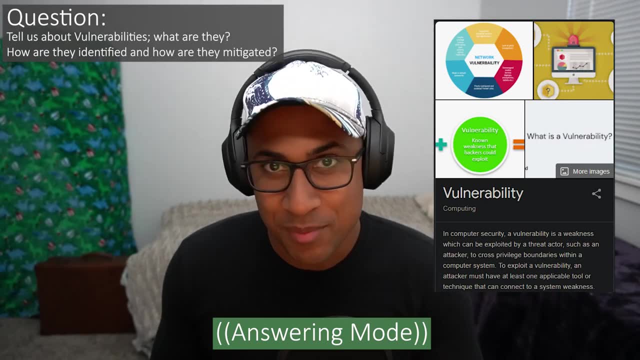 your home computer system, for example. um, your java is out of date. like to mitigate that. like either uninstall java or or update java. you know, set a password lockout policy or add a password. it just depends on on what the vulnerability is. one way to like mitigate vulnerabilities is to 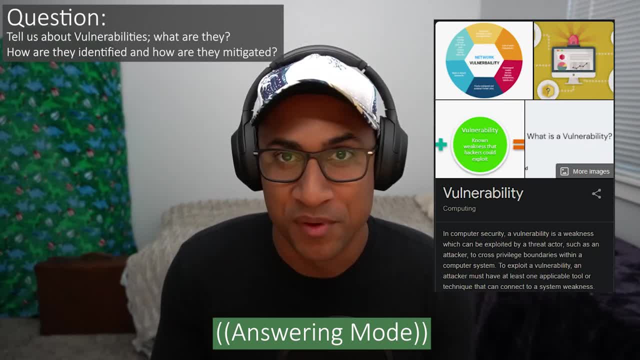 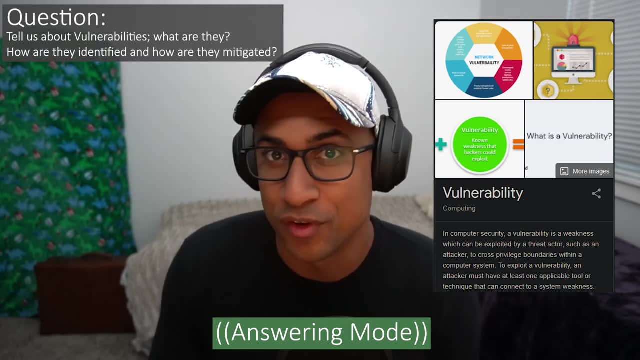 like remove the whole system altogether, right, like if your your home computer has java- like super old java- on it or something like this. technically you can remediate the vulnerability by like turning- never turning it on again. that's technically remediating it. but you know, of course, if you 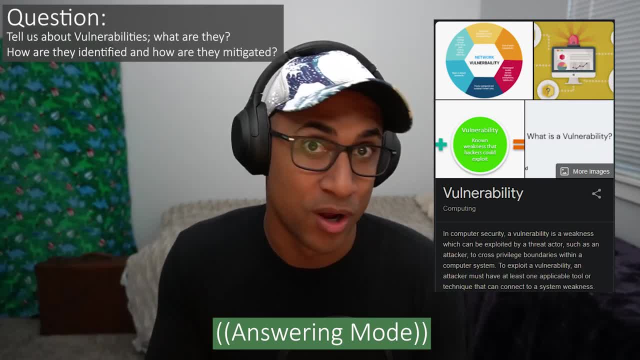 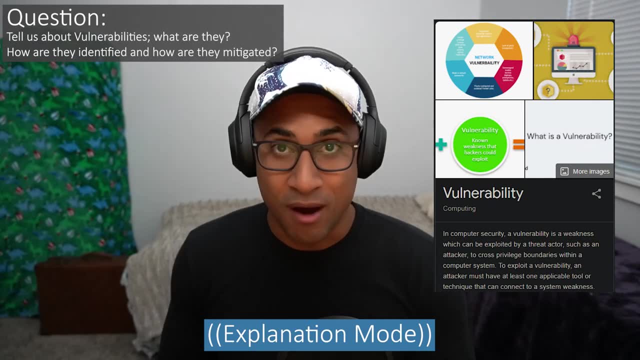 need the functionality of the computer. you have to, like you know, patch java or uninstall it, or something like this. yeah, so this question is pretty straightforward. um, just make sure you know what a vulnerability is and like be cognizant that they're not like only in the computer. they 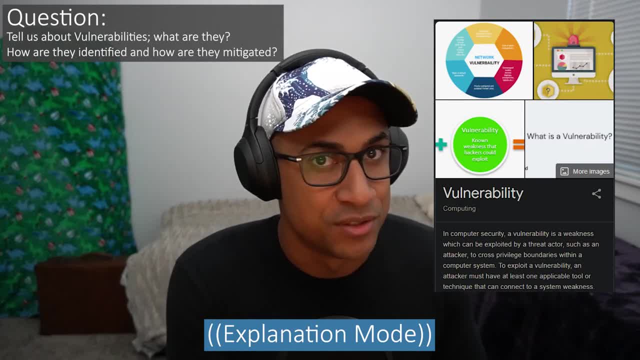 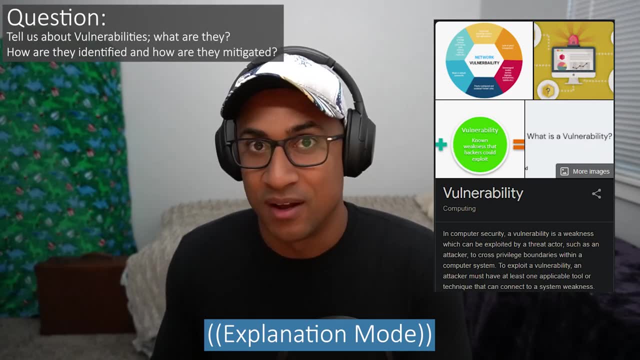 can be like a bad lock on, like a physical door or something like this or um. it can be like lack of process even, or like lack of policy or procedure, um, like, for example, if you, if you don't incident response plan, you haven't practiced it, that that in and itself can kind of be a 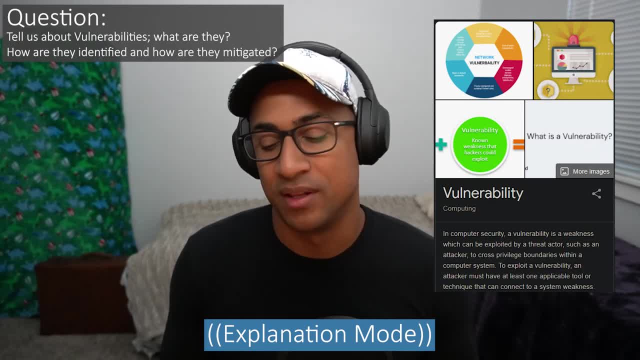 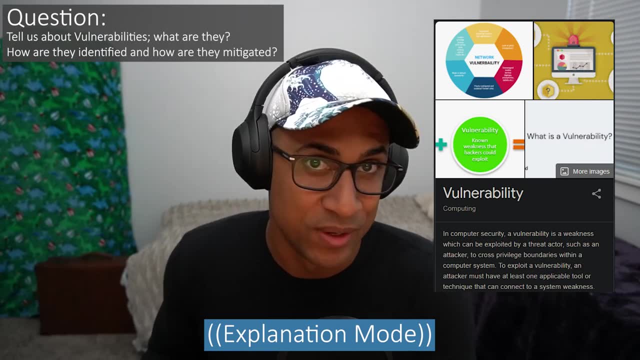 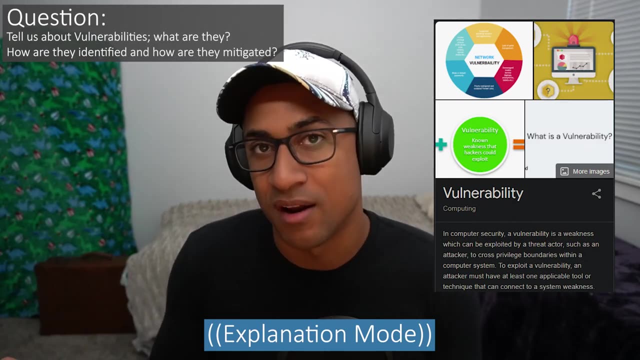 vulnerability because you won't be able to respond to incidents quickly enough, of course, those kind of traditional ones that everyone thinks about, like out of date software, poor os configurations, missing windows updates or missing os patches, these kind of things, and to mitigate them or to identify them, you know, use your eyeballs or just use some kind of automated software and then to 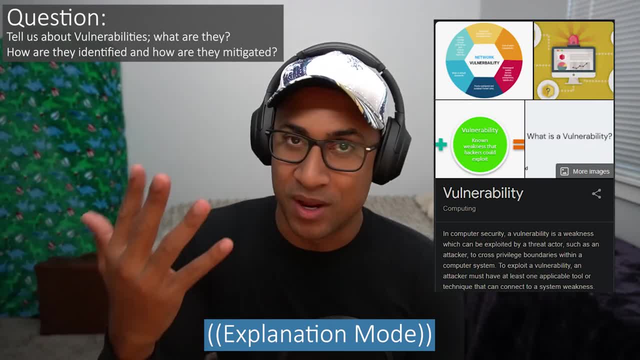 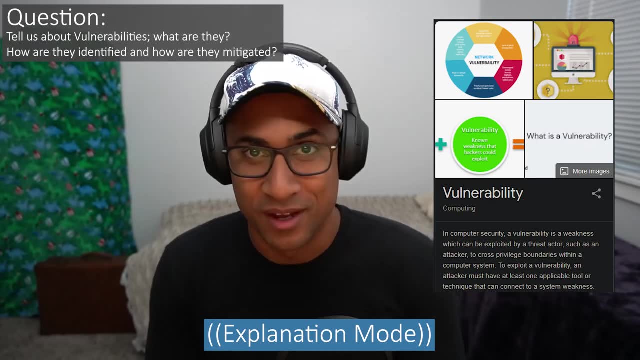 mitigate them. it just means, like, how to make them go away. so up, upgrade the locks, take the system and then just make sure that you have a good network. so that's a good question, important to understand. and the next question is: you are the only member of the information security risk and 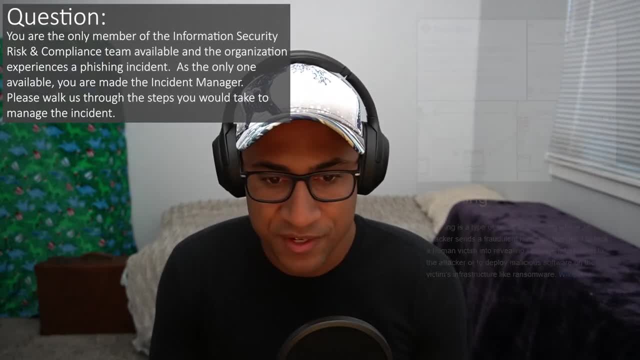 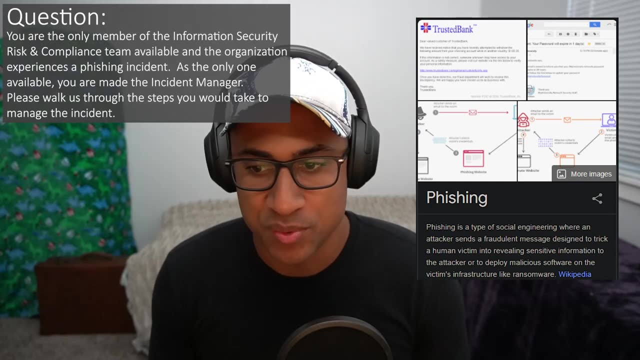 compliance team available and the organization experiences a phishing incident as the only one available. like being you, you are made the incident manager. please walk us through the steps you would take to manage the incident. so before i get into this, um, i just want to say, like, if there's a human, 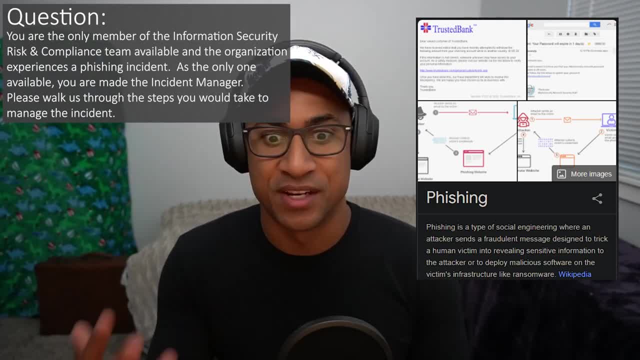 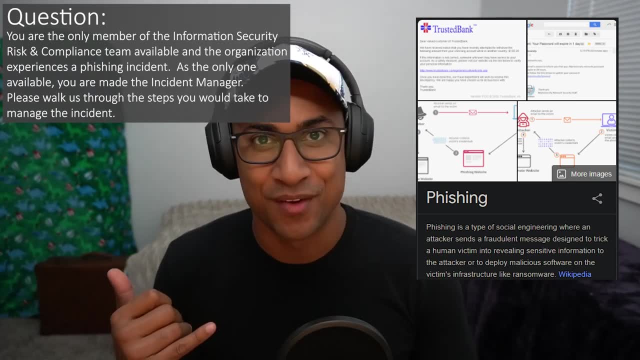 in front of me. i'd probably ask them more questions like: what kind of incident? like, what kind of what like? is it like a, an email campaign, or is it? is it like a phone kind of thing, like i don't know what it is? um, so i'm just going to answer this as if it were some kind of like email phishing campaign, and 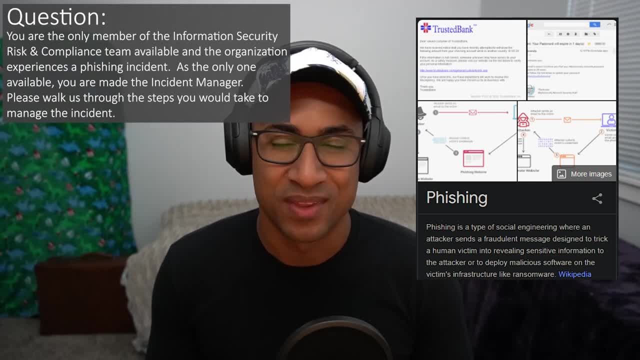 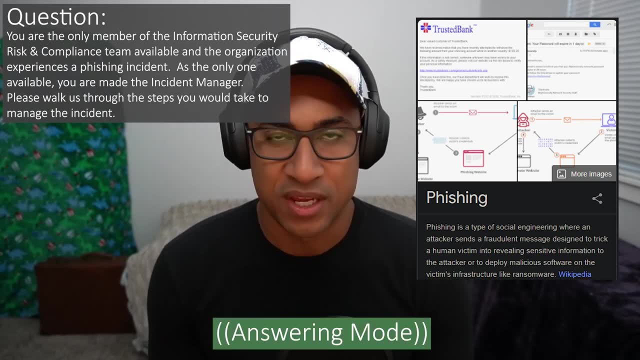 like there's. there's a lot more i could have asked to the human, like to the human interview, but i'll just do my best to answer. so if i was an incident manager for and we're in a phishing campaign and we had like that phishing incident, the first thing i would kind of do is i would verify that the, the 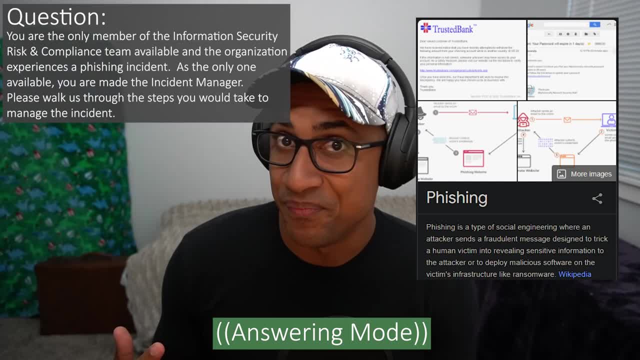 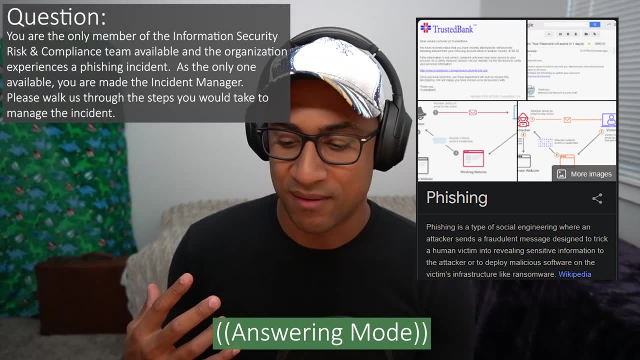 actually taken place. um, instead of, you know, maybe, maybe someone, maybe the ciso is performing like an actual campaign, where it's not like a real phishing person, it's a, you know, a simulated campaign to kind of get a baseline for the organization's awareness. but if i couldn't 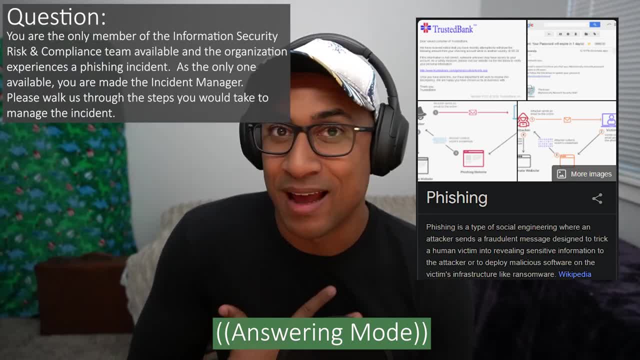 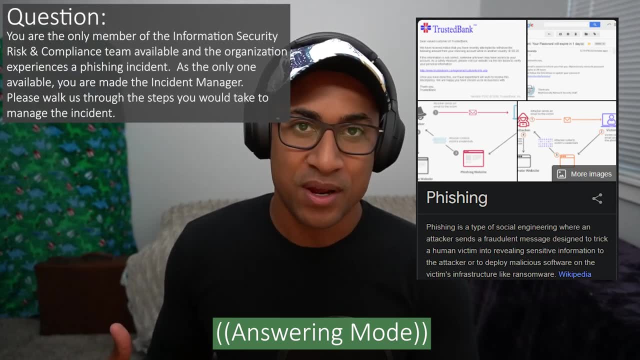 do that and i- i, you know, i was part of that, i was part of that experiment- uh, i would do my best to, like you know, of course, identify those happening and then try to contain it, uh, in some way, whether that is for, for example, if we have, like exchange, online protection or something i would try to like. 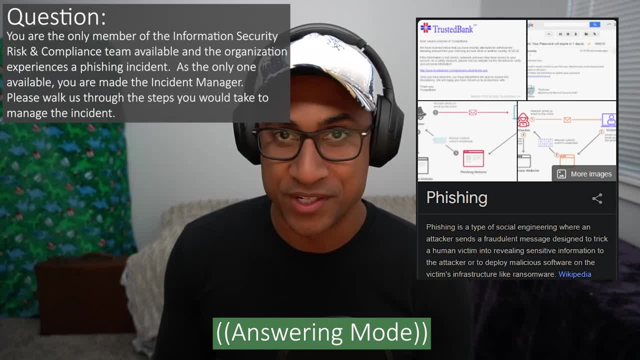 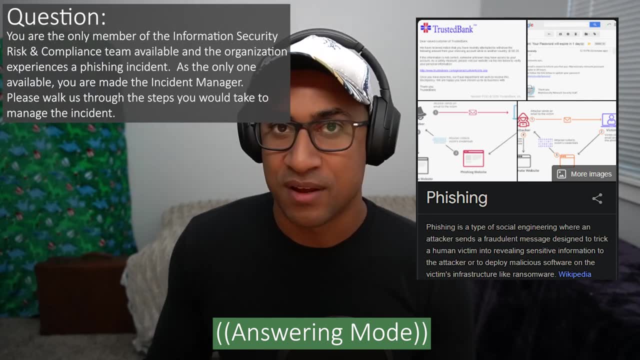 identify where the phishing campaign was like originating from, and try to further prevent that source from being able to send traffic into our network. and then for the stuff that was like already in the inboxes in our outlook or exchange implementation. i would try to go through and like: 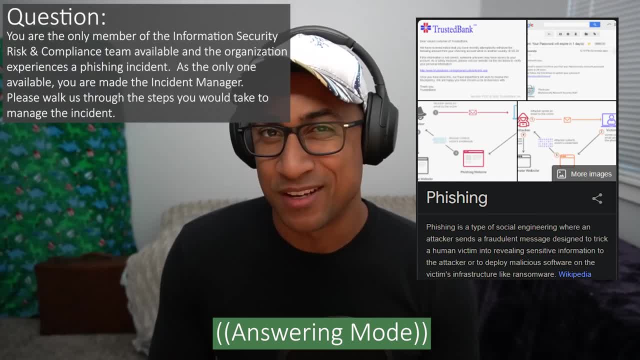 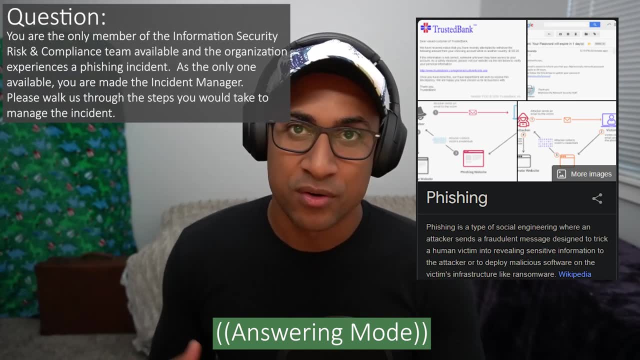 clean all of those out and then any of the computers, like depending on what was in the fish. if it was like a malicious link or something, i would identify the phishing campaign and then i'd identify, like kind of all the users who were targeted, who, like either opened it or had it sent. 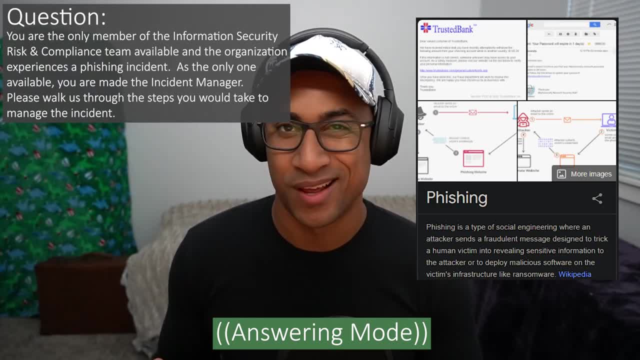 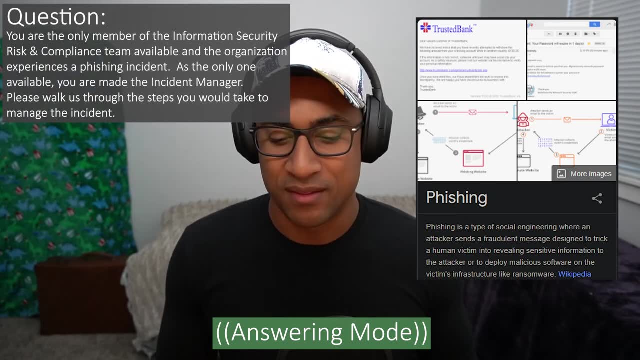 to their inbox and i would take their, their workstation, offline again, depending on like what was actually in the fish. so, as part of the, the containment part, you know, identify the the scope of what had happened and remove it from the inboxes and take those people's computers offline. 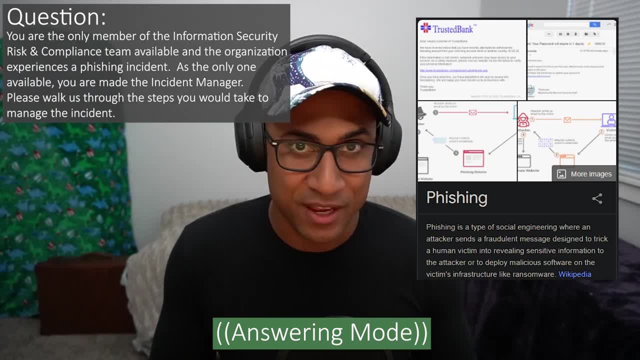 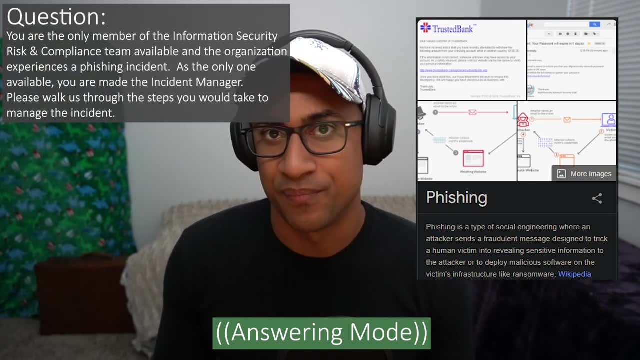 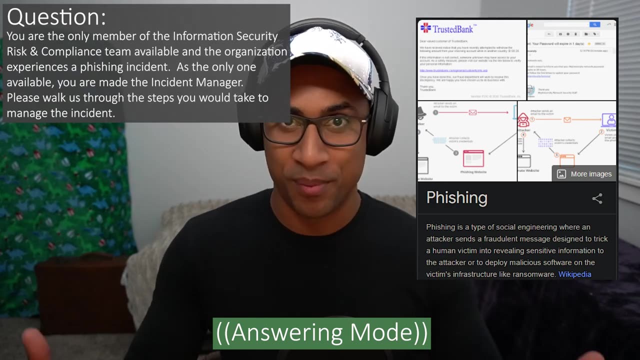 and the next step i would kind of go into like the maybe like the eradication phase. in case any there was malware involved, all the computers that we took offline of the targeted people. we'd go ahead and um wipe those and re-image them, kind of verify that the kind of reached the scope of. 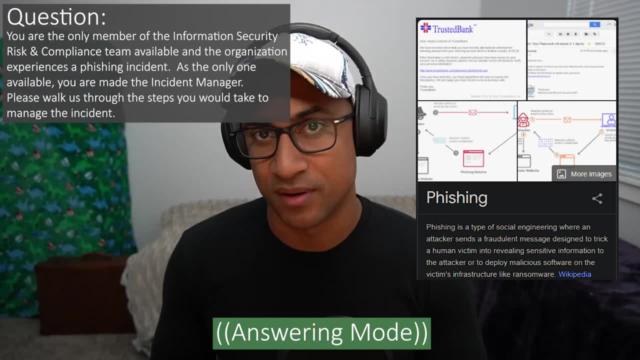 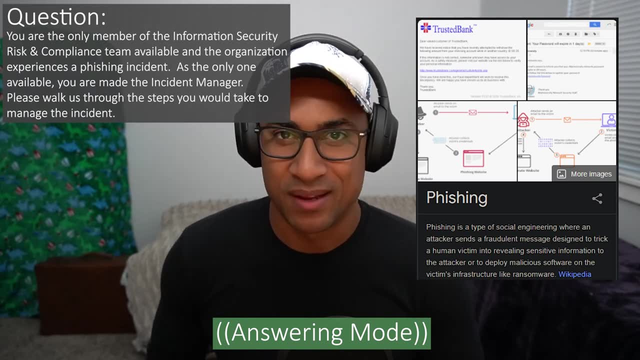 everyone that was kind of involved and make sure to like re-image all of their, all their uh computers, clean up any, any malware that could have happened, and once we kind of determined that everything was cleaned up and we were no longer kind of receiving uh the phishing from whatever, 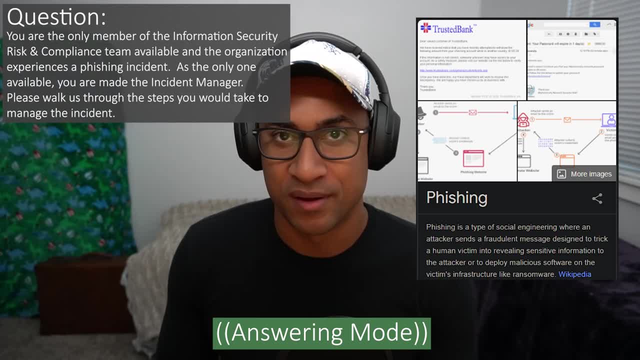 the source was put the new computers back online and we'd kind of have a like a post-mortem meeting where we kind of see if we can learn anything about what happened and kind of reform our incident response process a little bit if we have to, and just kind of um do what we can to make. 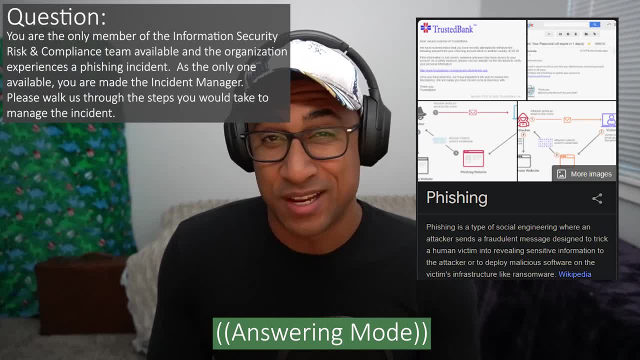 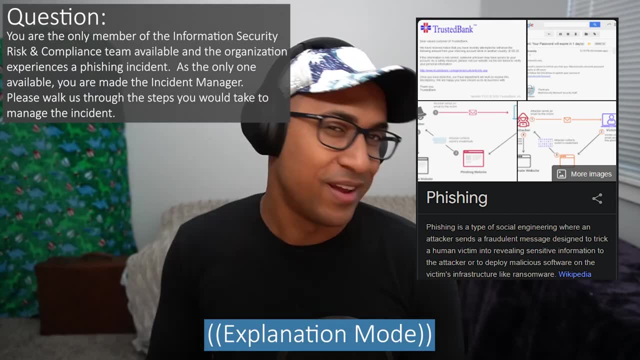 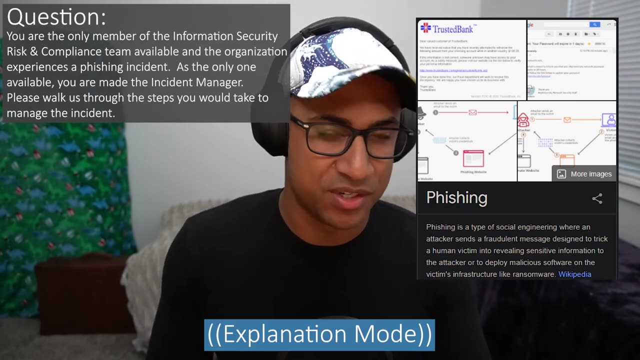 us be able to handle the situation like better in the future. so this is like a really hard question. um, i don't know if there's necessarily a correct answer to it, but i i tried to. i tried to answer it in line with, like the, the nist, 861, i believe, like the computer incident. let me, let me just like look. 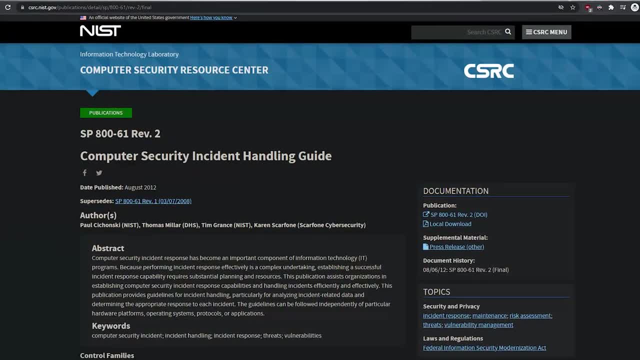 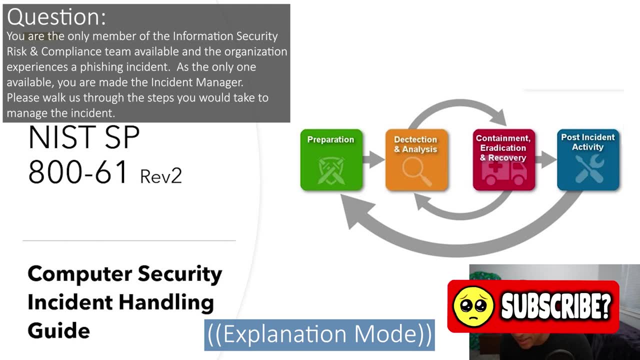 it up really quickly here. oh, the computer incident handling guideline kind of has like certain steps that you, that you follow for like an incident, for example, like preparation, detection and analysis, containment, eradication and recovery and then kind of post incident activity. so i kind of touched on. 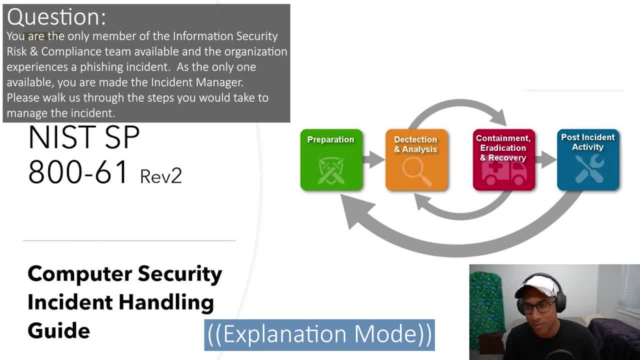 most of these things. i didn't talk about preparation because i guess the incident was already happening, but detection and analysis. um, detection, like make sure that it's actually happening, and analysis kind of determine the scope of it and see if there's like any kind of malware involved that might have affected any of your computer systems, and then like containment. 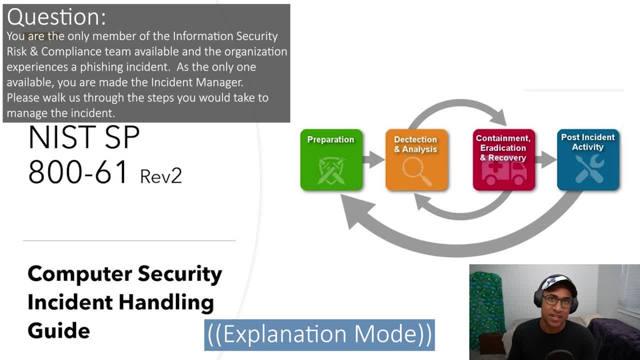 eradication and recovery: containment right. block the sender from like sending more, take the computers offline that got infected. eradication like: re-image the computers that potentially got affected. recovery like: uh, i guess that's eradication and recovery. it would be like, you know, wiping the computers and re-imaging them. and then i kind of talked about the post-incident. 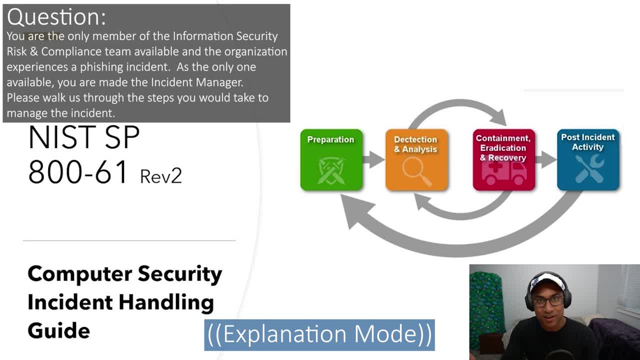 thing i tried to. i tried to like describe this off the top of my head but i couldn't very well, but maybe it matched like a little bit. if someone gave me the answer that i just gave, i'd be like, okay, they, they know what like nist 861 is, or at least they're familiar with, like the incident. 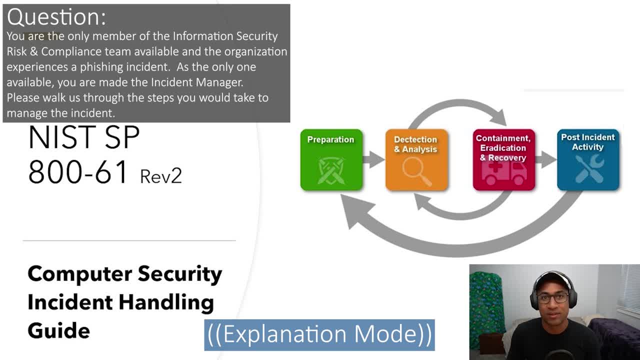 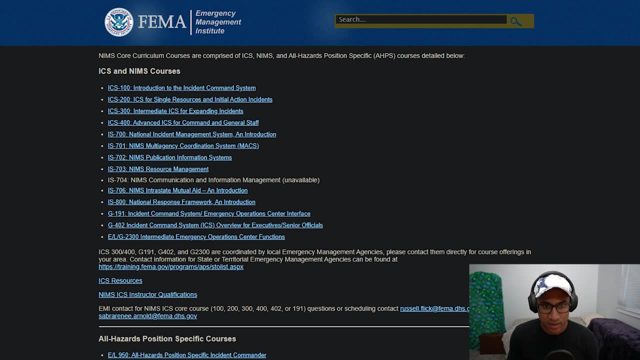 um, kind of the incident handling process at a high level. so i would look up like uh, nist 861, and then you can even there's like some free training online. let me look it up that you can do to kind of put on your resume. even it's uh, the fema training, like ics. 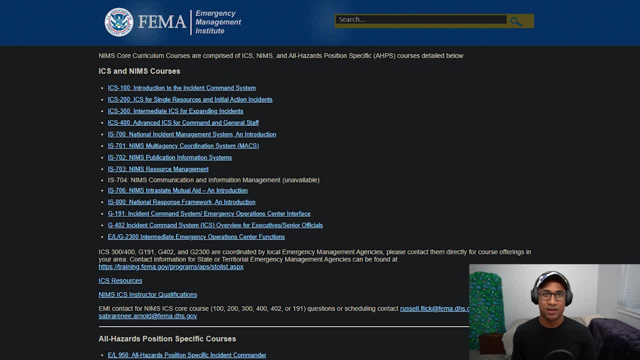 so google like fema, fema, ics, 100, it's kind of like a figure. what ics stands for incident command system, it's kind of like an incident handling thing and you can get a certificate and you can like put it on your on your resume. so yeah, nist 861 and then fema, ics, kind of you know digest.